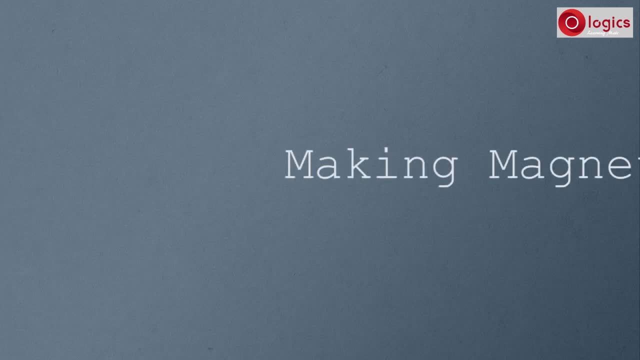 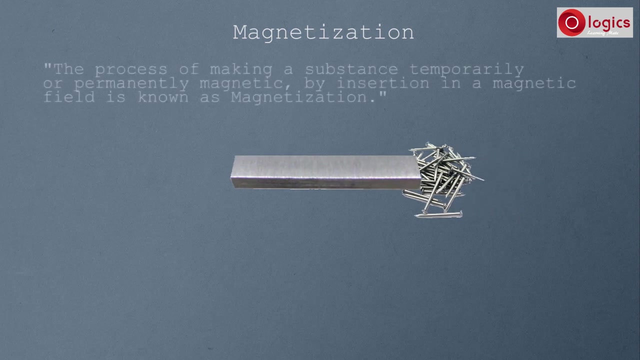 Let's see how to make magnets. Any magnetic material can become a magnet by magnetization. This is a steel substance. Observe this: steel substance is not a magnet. With some process or method, this steel bar can be made into a magnet. The process of making a substance. 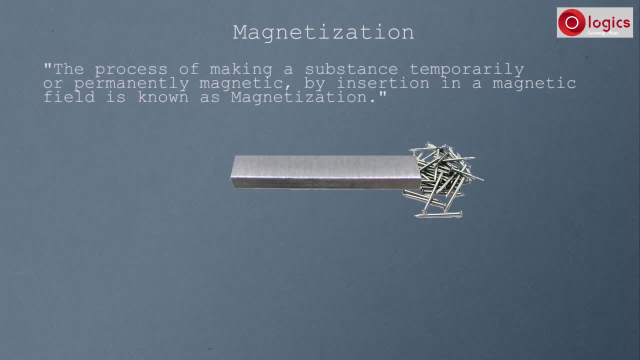 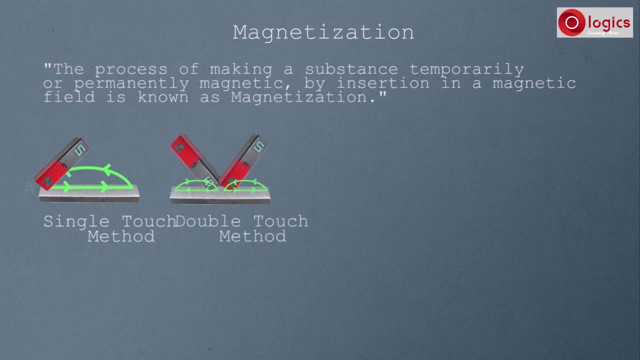 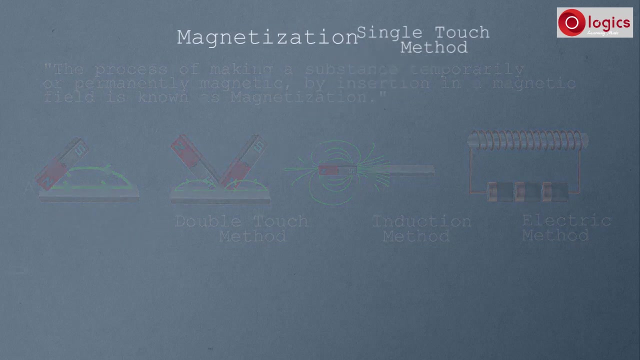 temporarily or permanently. magnetic by insertion in a magnetic field is known as magnetization. There are four methods of making this steel bar into a magnet: Single touch method, Double touch method, Induction method, Electric method. Let's see what is single touch method. This is the steel bar, This is not magnet. now, 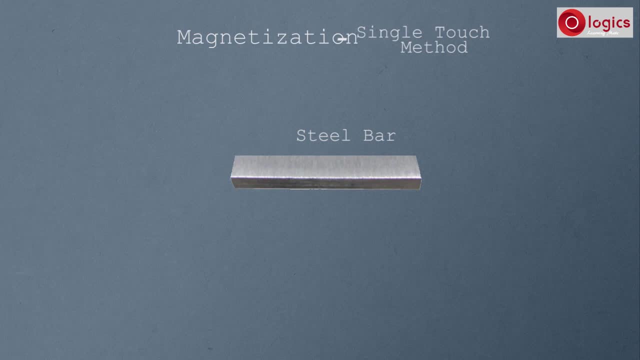 Here I am going to make this steel bar as a magnet by adopting single touch method. Let this end is A and this end is B of this steel bar. This is a magnet. This is the north pole and this is the south pole of the magnet. 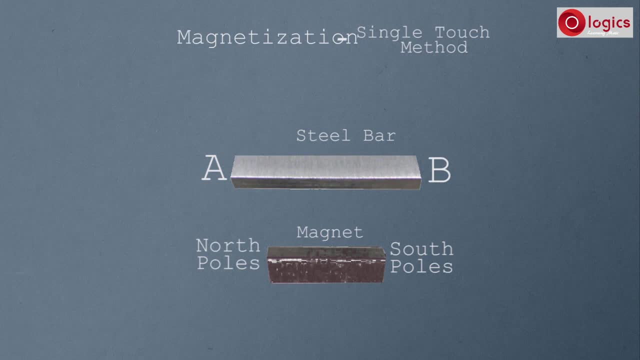 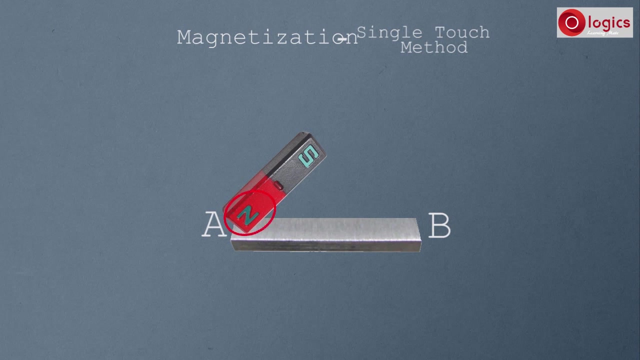 For identification purpose, usually artificial magnets, north pole colored as red and south pole colored as black In single touch method. Hold magnet at end A of steel bar like this, With north pole of magnet touching steel bar. gently rub steel bar from end A to end. 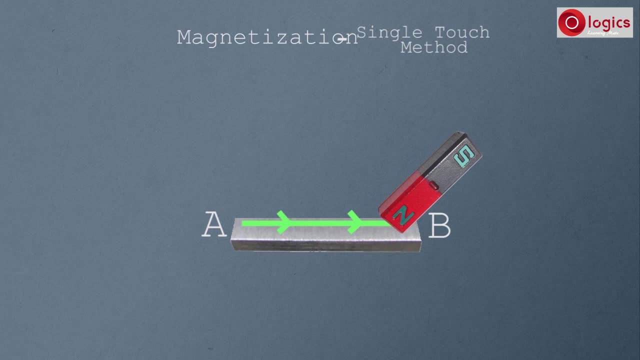 B like this. Now lift up magnet and bring magnet to end A like this Again. rub steel bar from end A to end B. Repeat this process several times. After rubbing for many times, end A of steel bar becomes north pole & end B of steel bar. 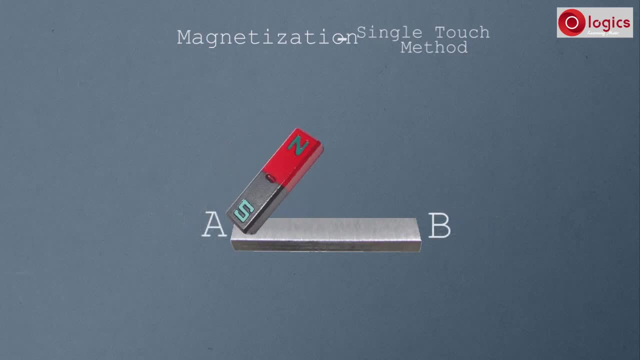 becomes south pole. Now you can night watch this video. Like, like, share. like by hitting like button. Thanks. of magnet is used to rub steel bar, then n a of steel bar becomes South Pole and end B of steel bar becomes North Pole. now this steel bar became magnet. let's 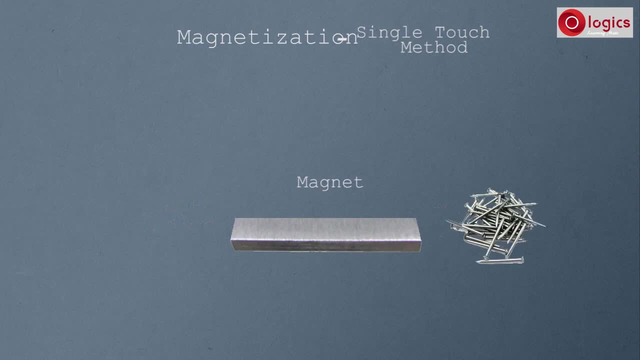 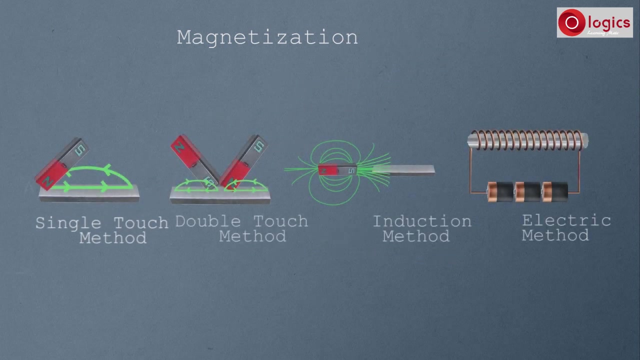 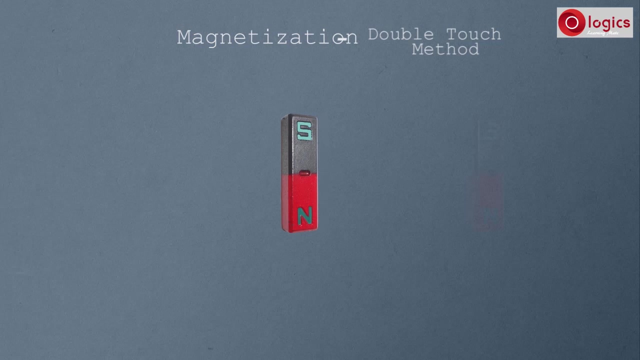 test this magnet. take iron pins, and these pins are attracted by steel bar, which became a magnet. this time, let us magnetize substance using double-touch method. in single-touch methods, magnetization done with single magnet. now, in double touch method, we need two magnets. let us see how to magnetize this magnetic substance. 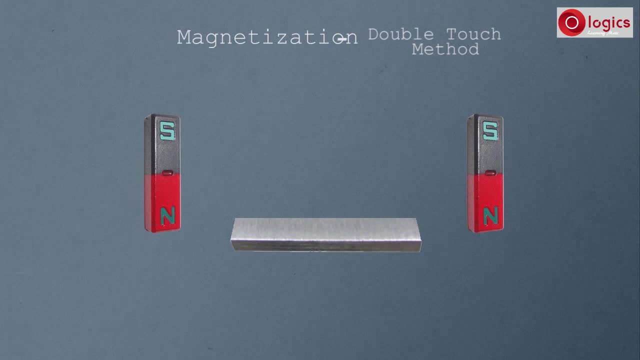 steel bars bar. Let. this end is A and this end is B of this steel bar And C is the center of magnet. Lift up magnet. Hold both magnets at central, With south pole of this magnet touching steel bar And north pole of second magnet touching steel bar. 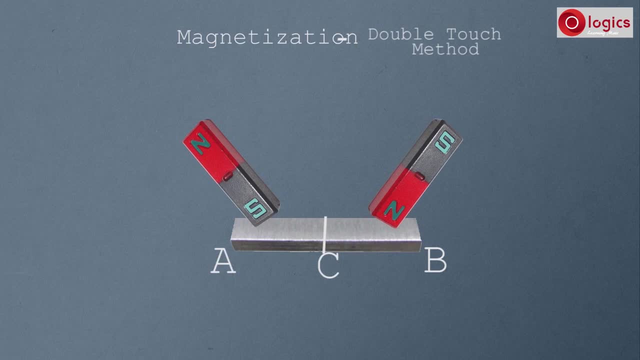 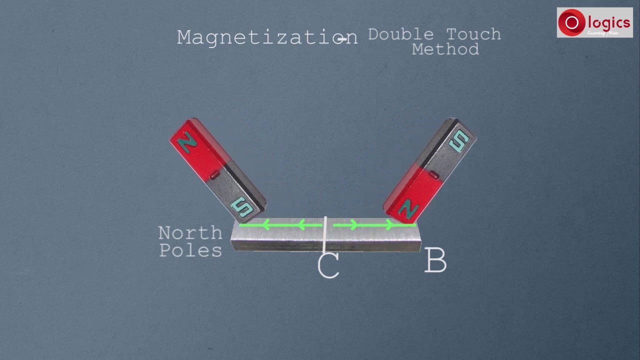 From center C. rub both magnets like this At ends A, B, lift the magnets and bring both magnets to middle again. Repeat this process for many times, Since end A is rubbed with south pole of magnet To end A becomes north pole And end B is rubbed with north pole of another. 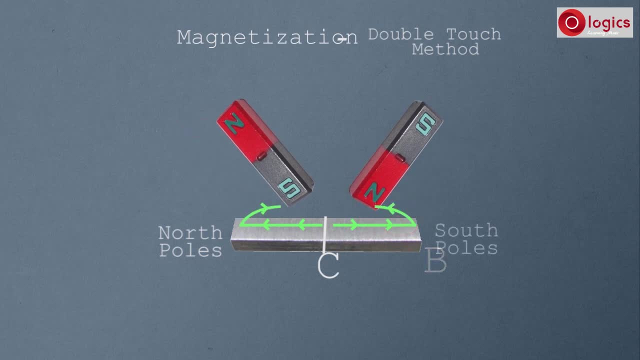 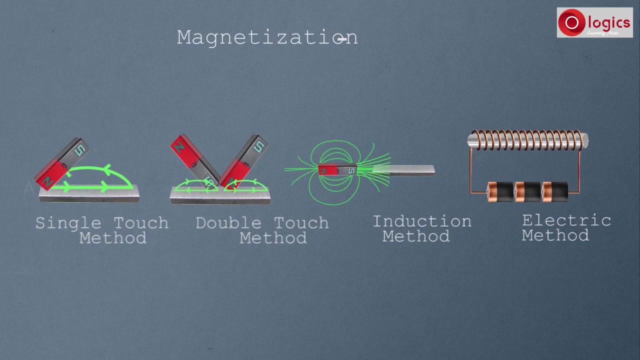 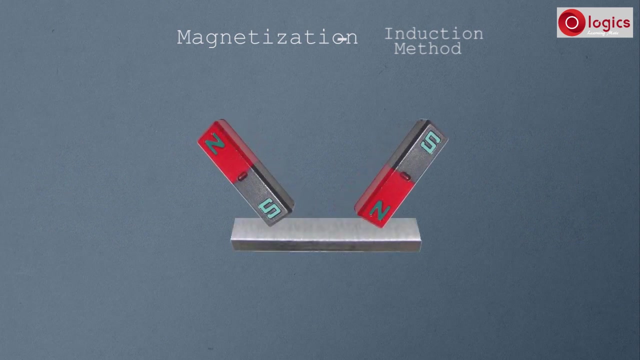 magnet. End B becomes south pole. Now this steel bar became magnet. This is double touch method of magnetization. This time, let us magnetize substance using magnet. This time, let us magnetize substance using magnet. This time, let us magnetize substance using magnet induction method. till now, we rubbed magnets with steel bar to make it. 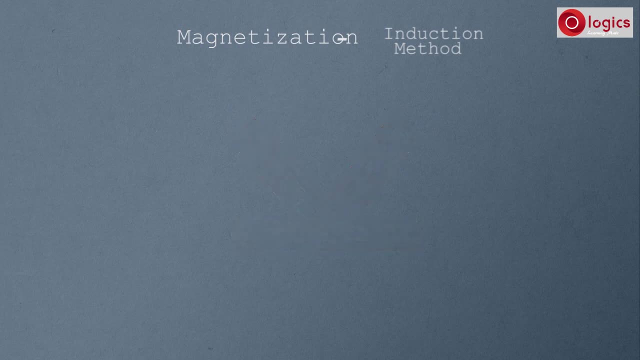 magnet in induction method. steel bar is made into a magnet without any contact. let us see how to magnetize this magnetic substance, steel bar. let this end is a and this end is B of this steel bar. this is a magnet and this is its north pole and this is. 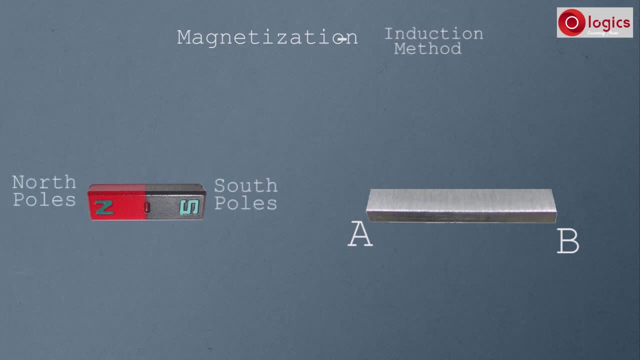 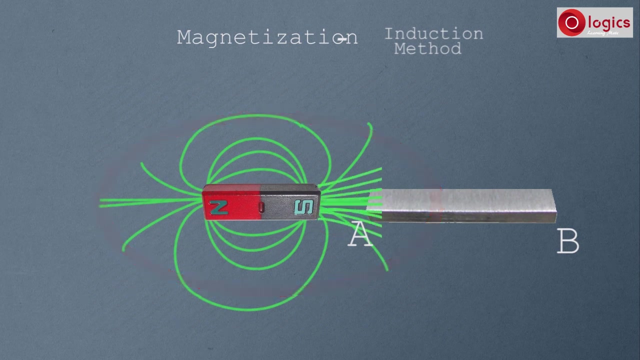 South Pole. now place South Pole of this magnet, side to side, two steel bars a end. observe magnet and steel bar are not touched but But steel bar is in magnetic field of magnet. Due to this, magnetic lines of force passes through steel bar. After a while observed, steel bar becomes a magnet. 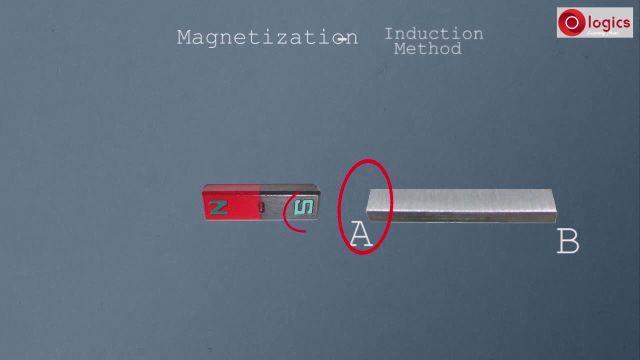 End A, which is side by side to south pole, of magnet, became north pole, And end B, which is away from south pole of magnet, became south pole. Now this steel bar became magnet. For better induction method of magnetization, following factors are to be considered: 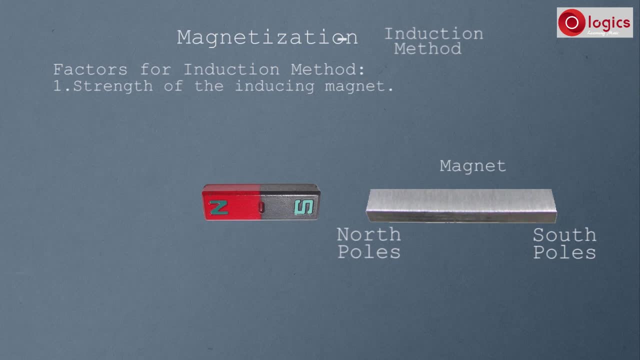 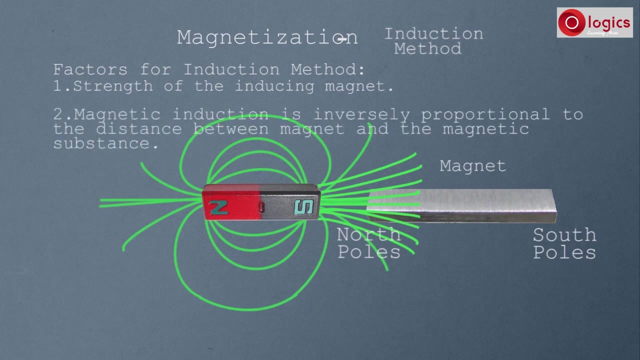 First, strength of the inducing magnet. This magnet should be more powerful So that more magnetization. Second, magnetic induction is inversely proportional to the distance between magnet and the magnetic substance. If this distance is less, more magnetic field is induced into substance. 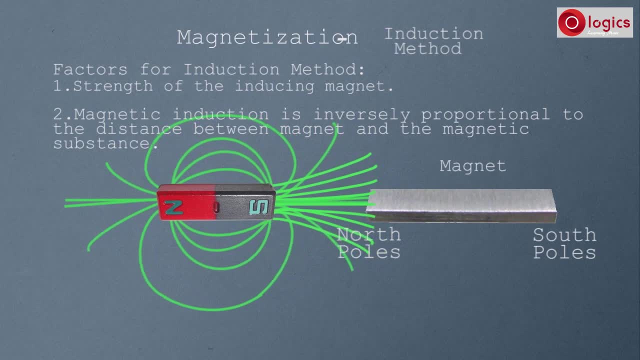 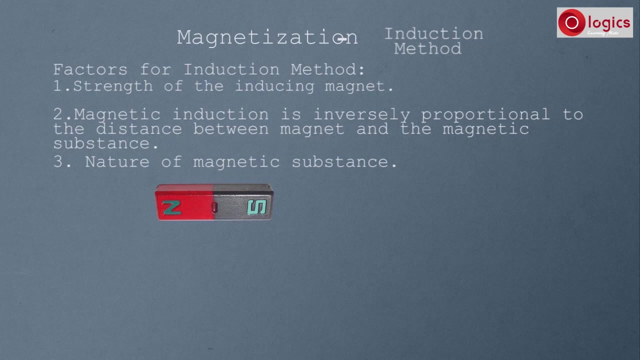 If distance is more, less, magnetic field is induced into substance. Third, Nature of magnetic substance. Permanent magnetization depends on nature of magnetic substance. Let us take two types of magnetic materials. One is steel and other is soft iron. If the magnetic substance is steel, 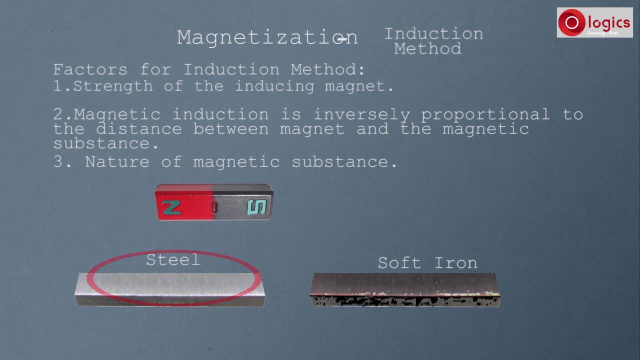 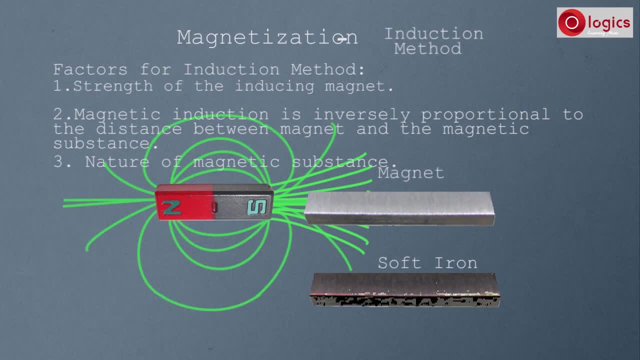 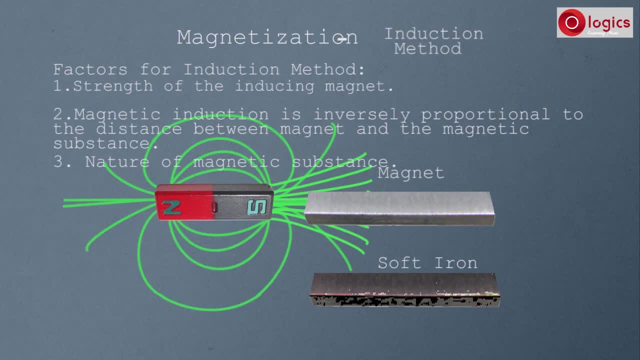 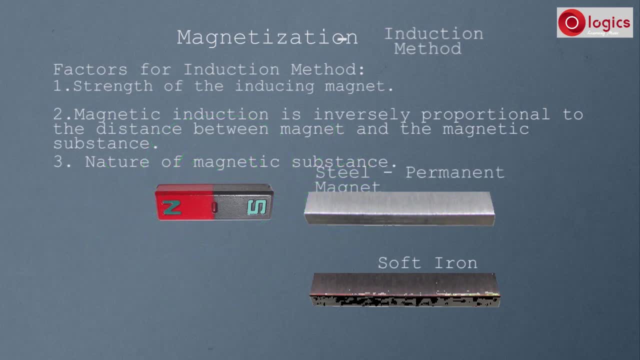 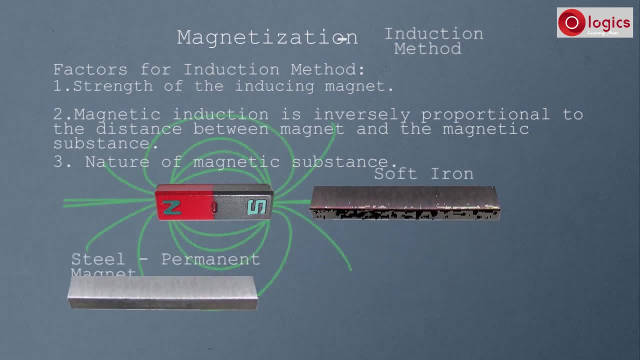 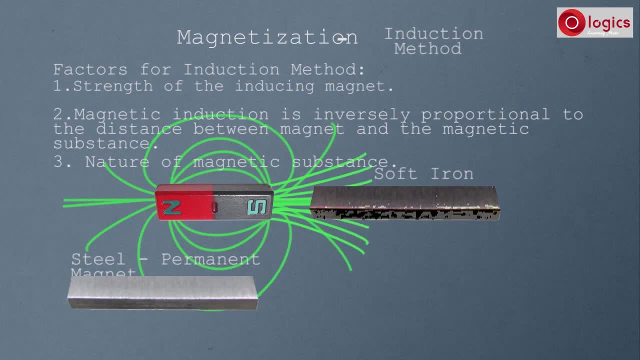 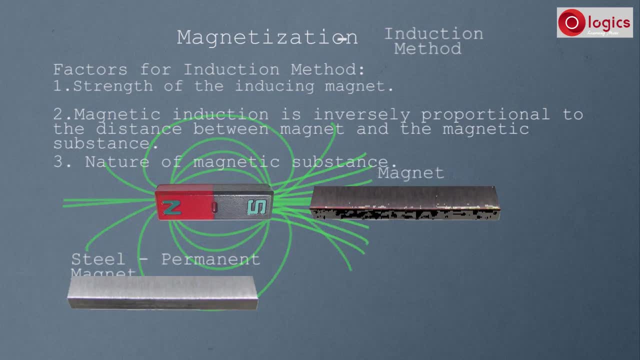 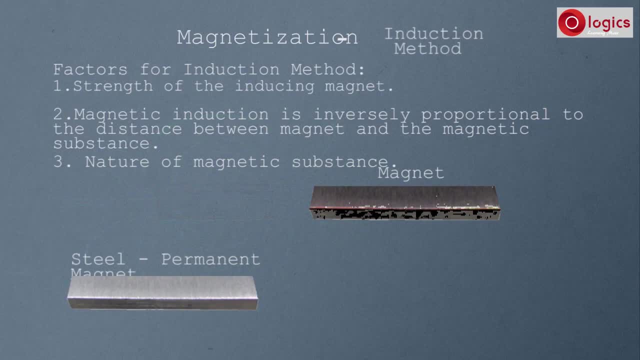 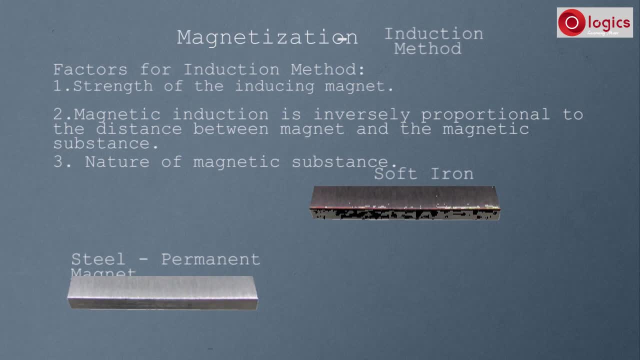 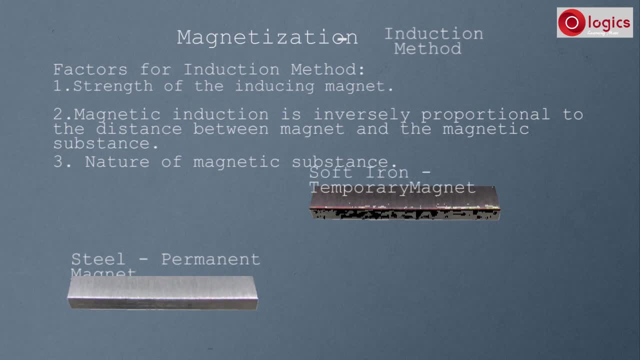 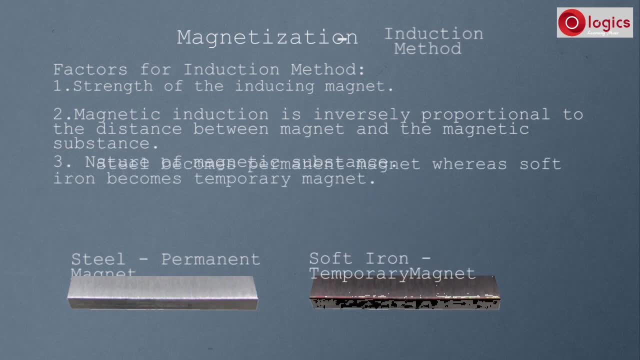 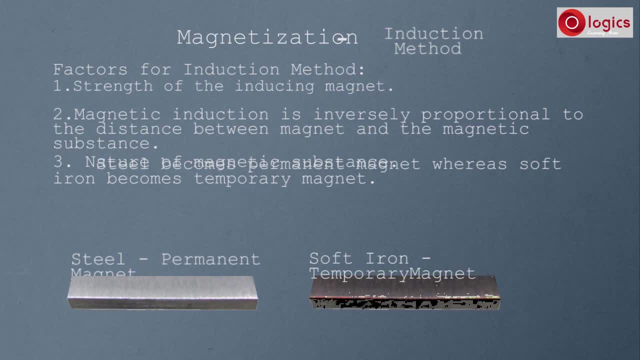 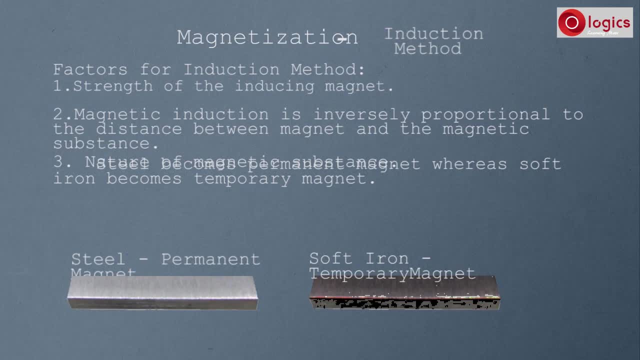 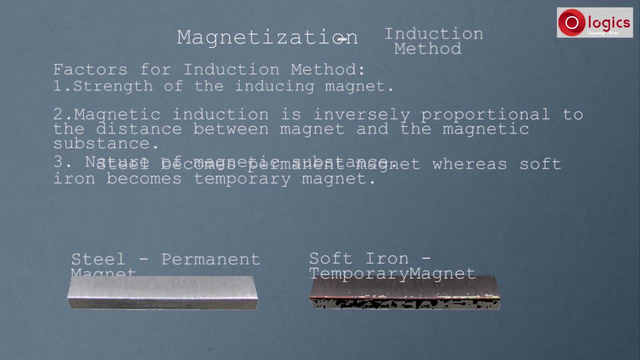 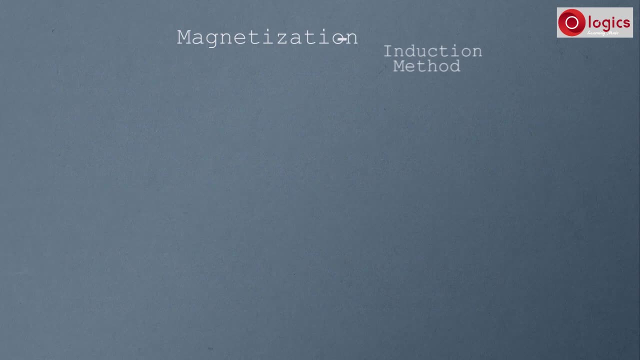 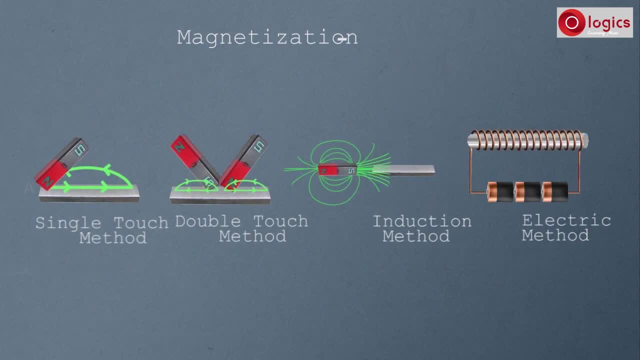 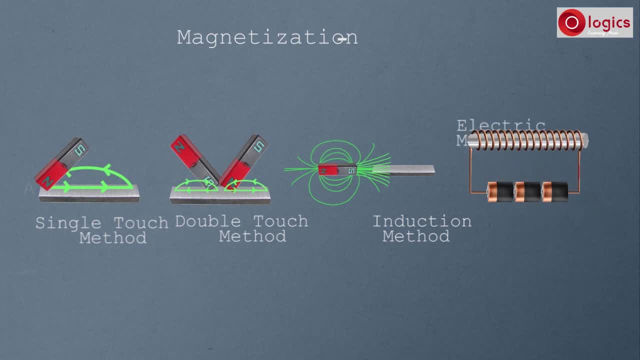 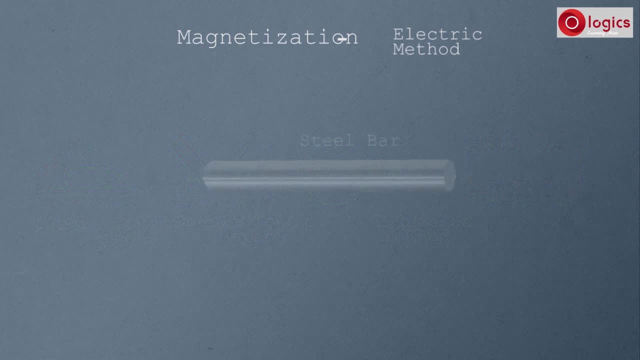 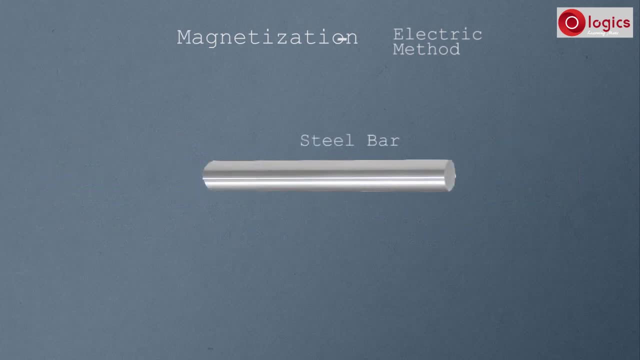 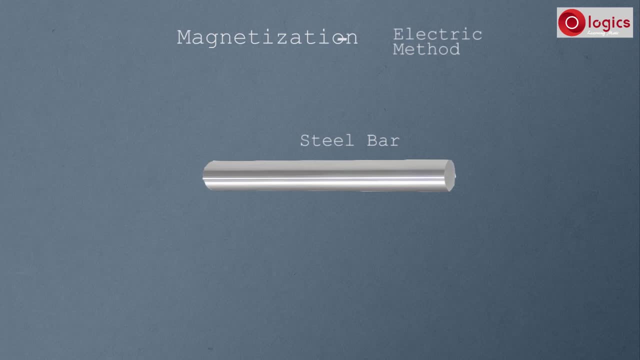 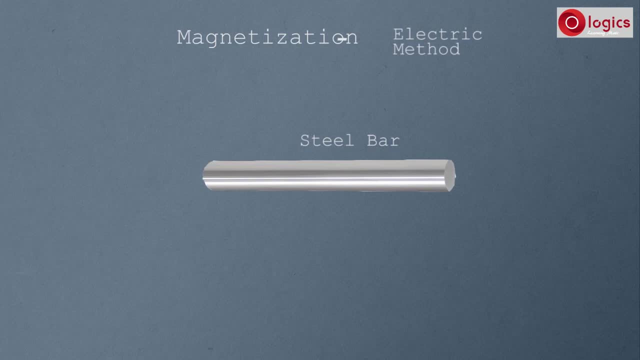 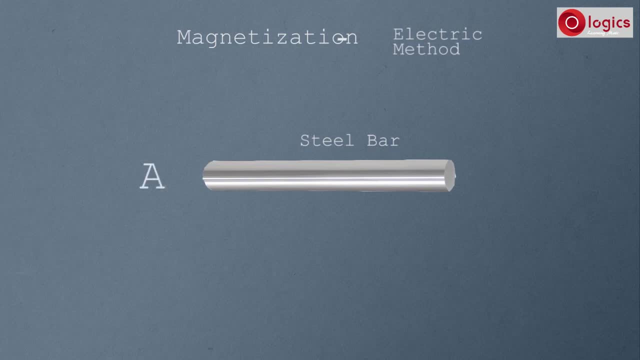 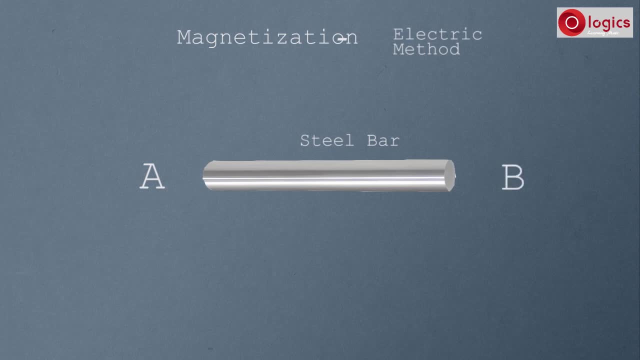 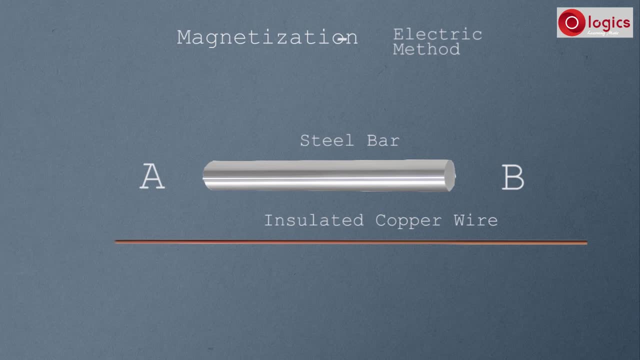 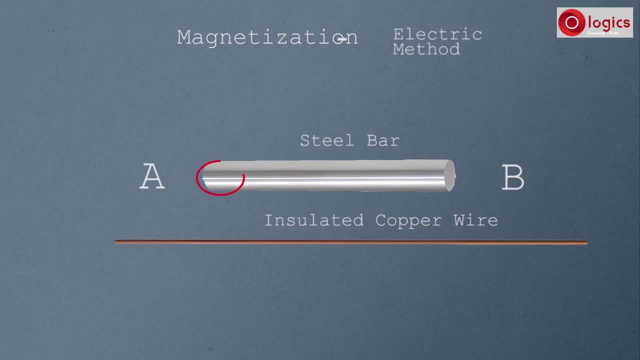 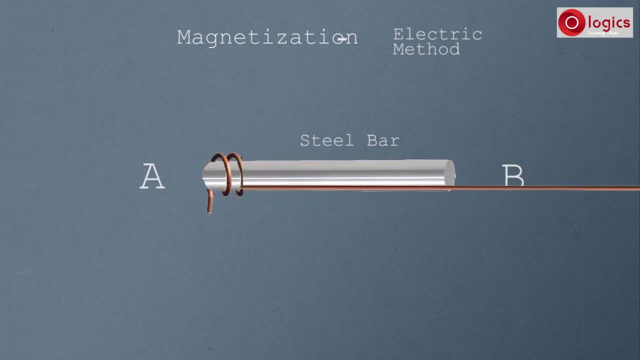 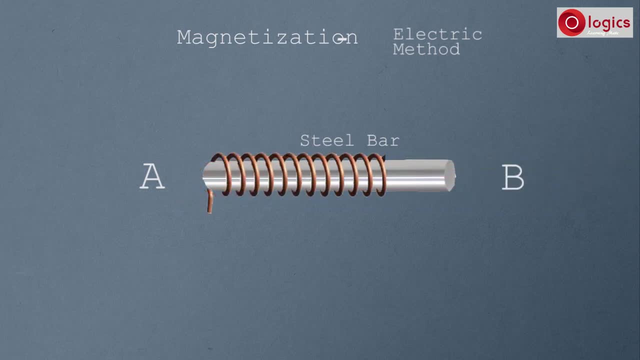 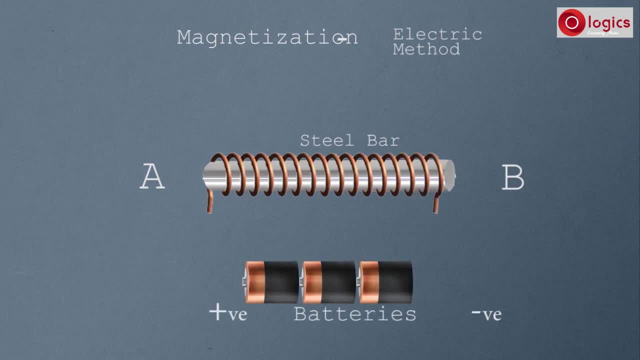 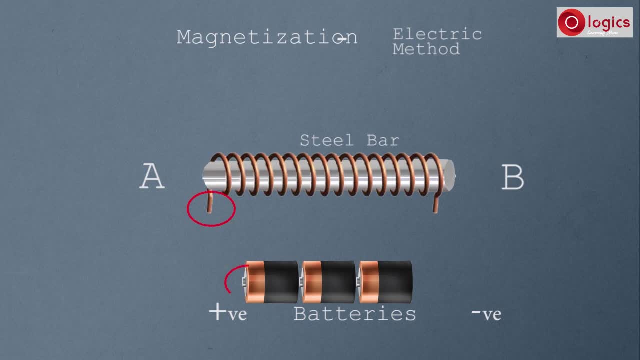 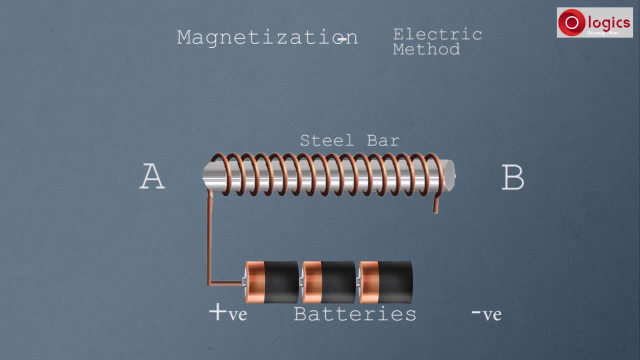 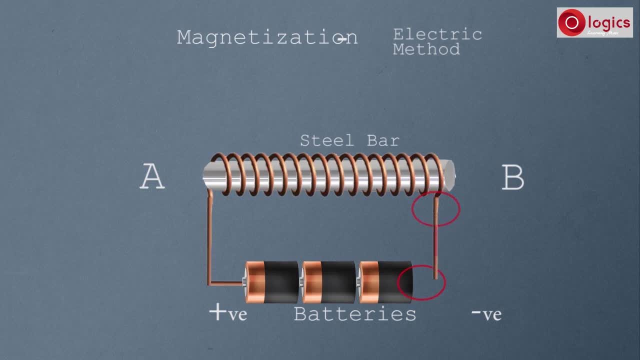 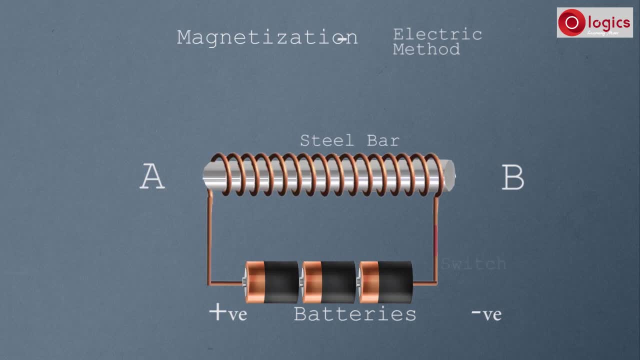 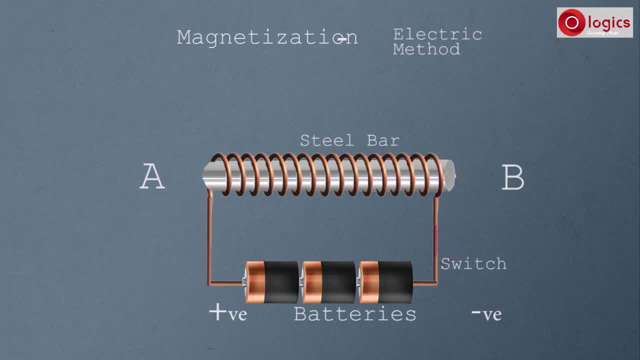 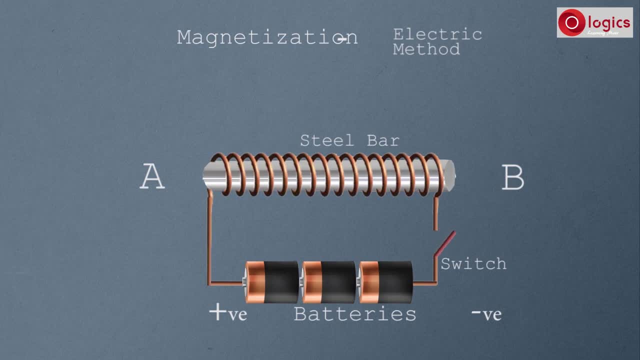 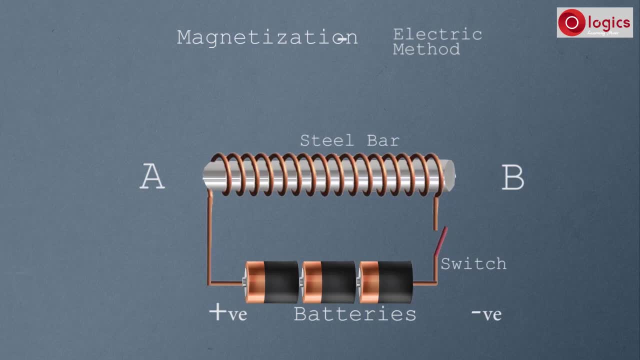 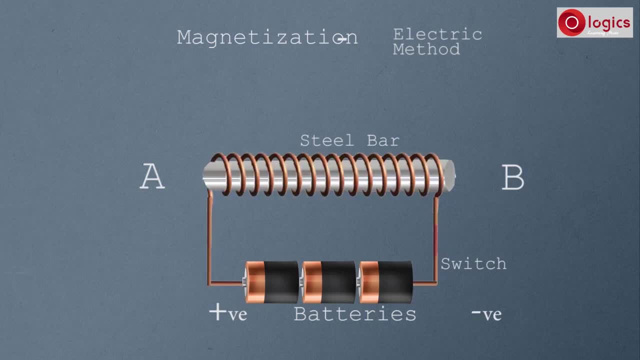 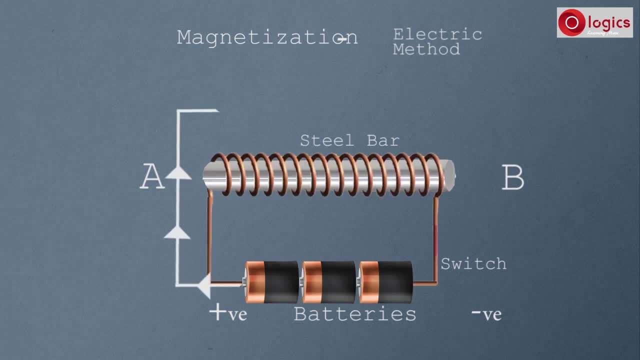 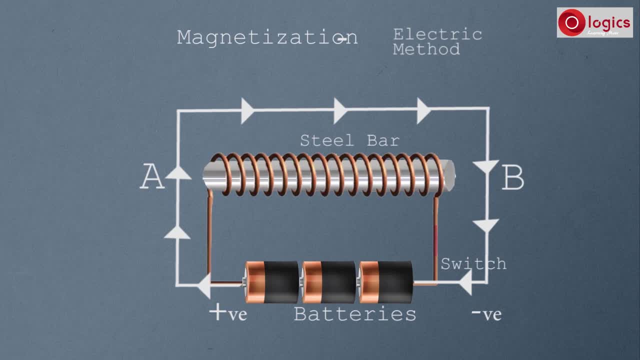 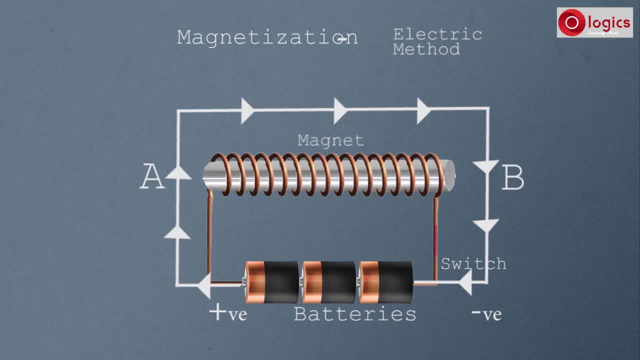 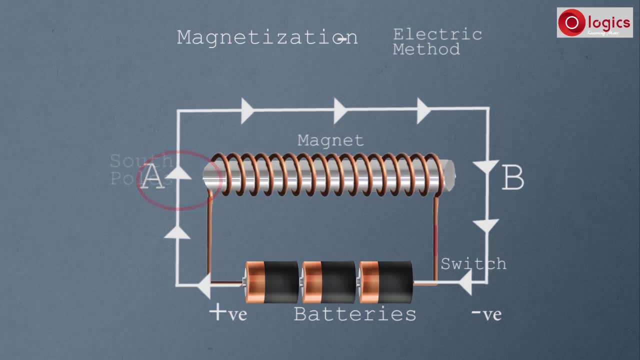 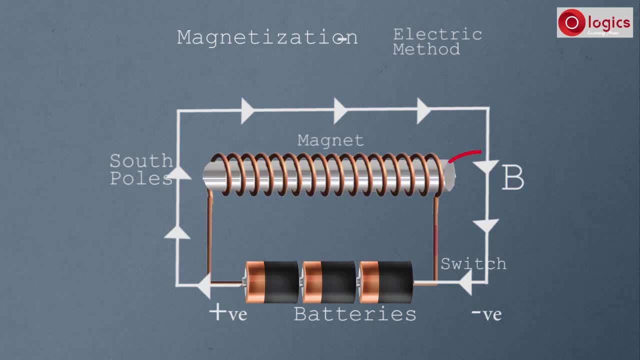 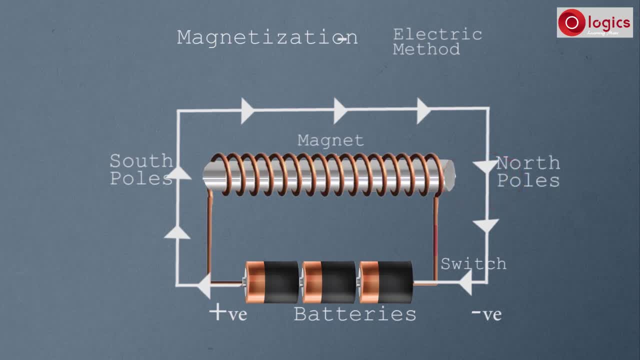 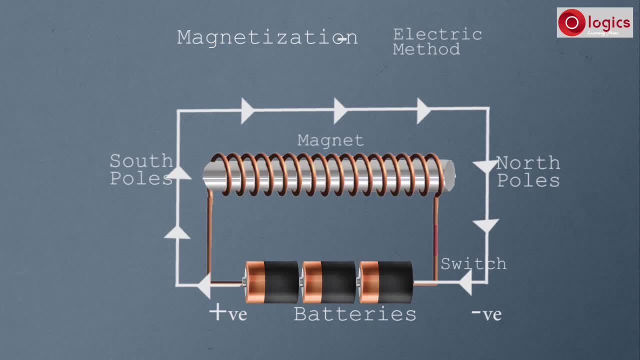 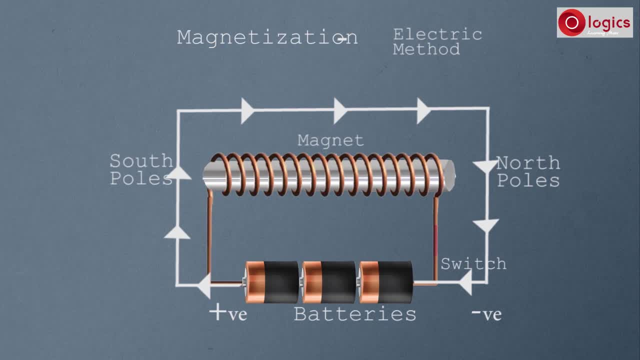 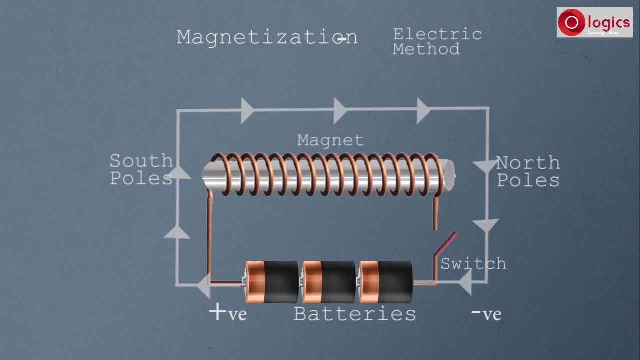 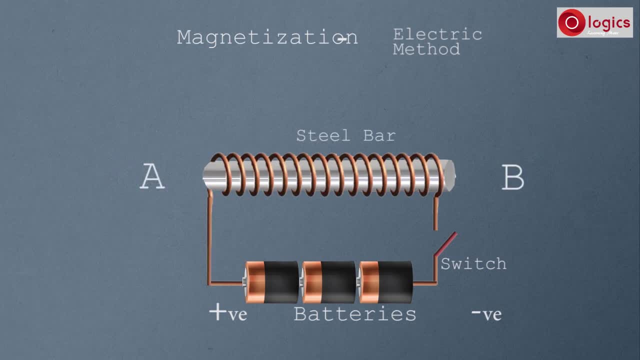 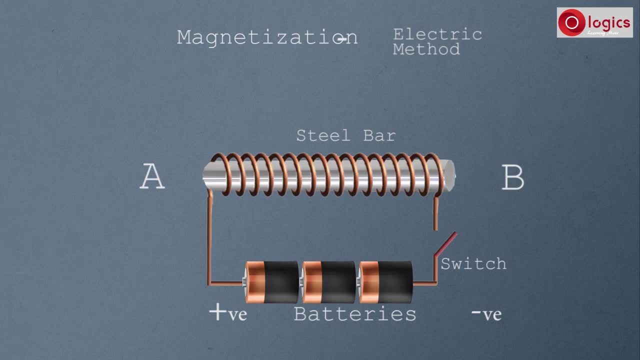 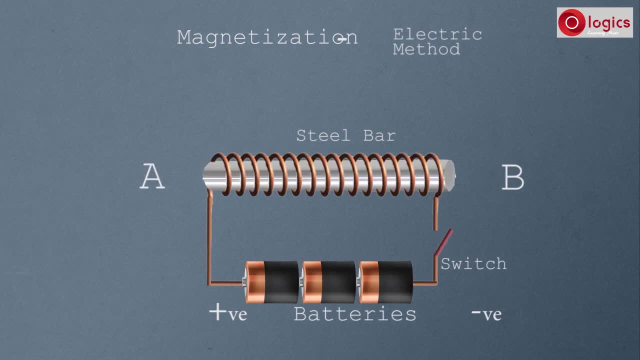 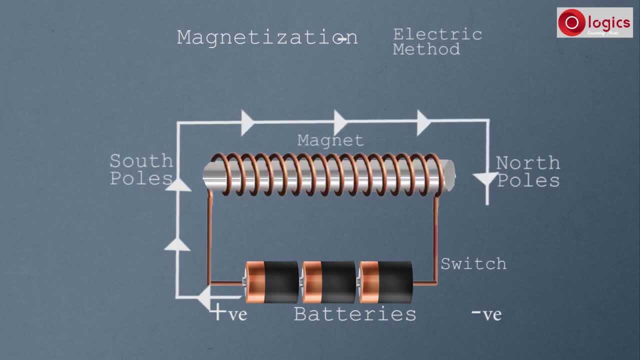 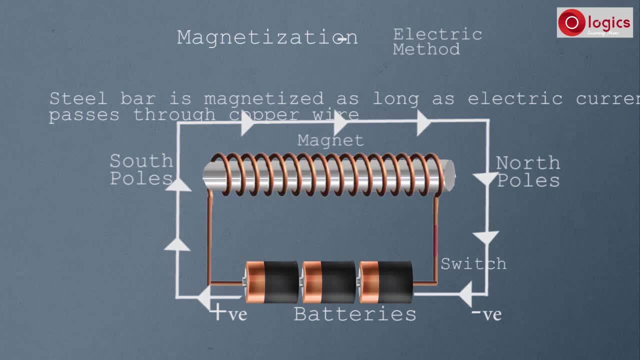 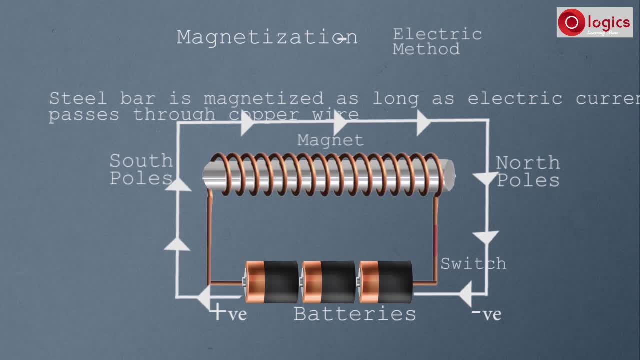 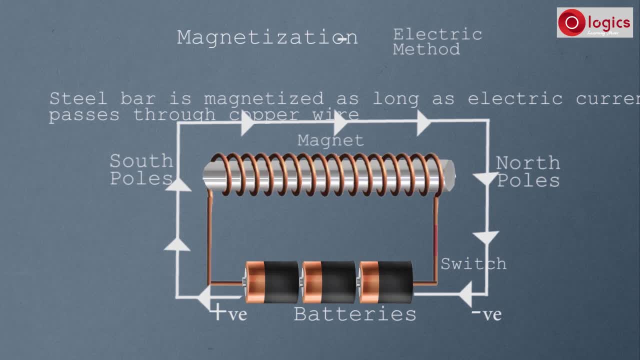 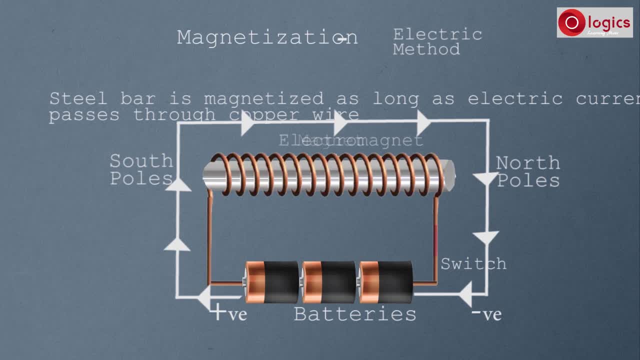 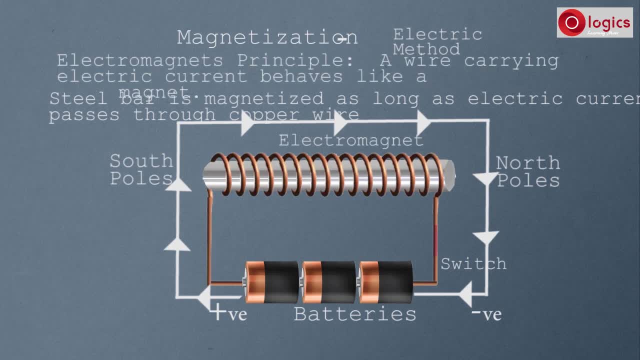 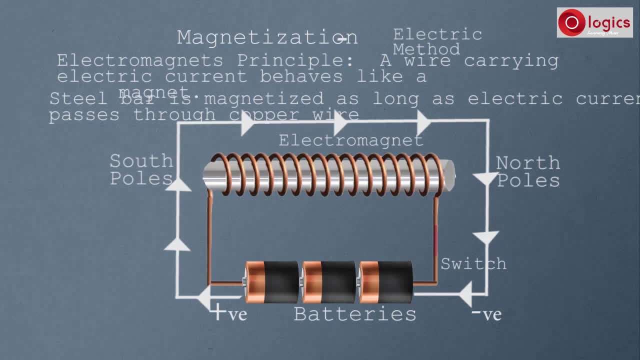 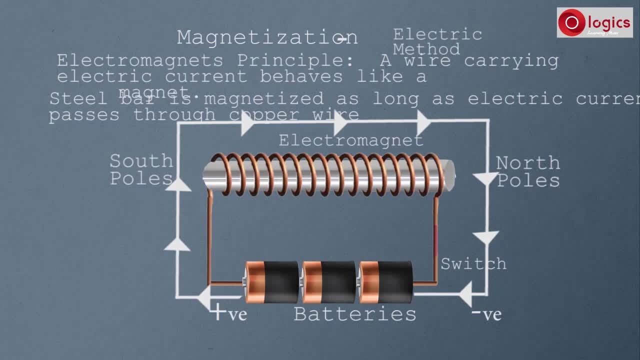 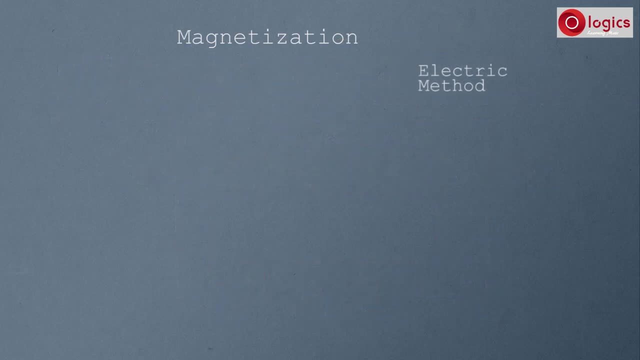 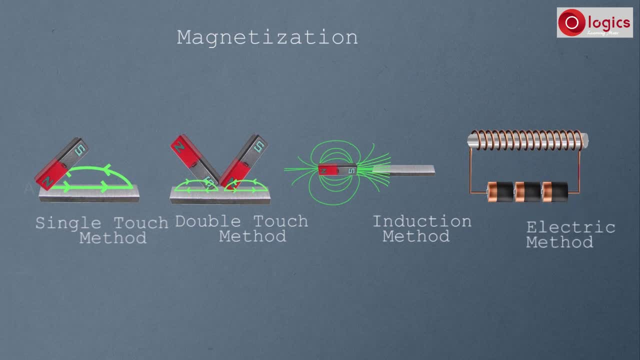 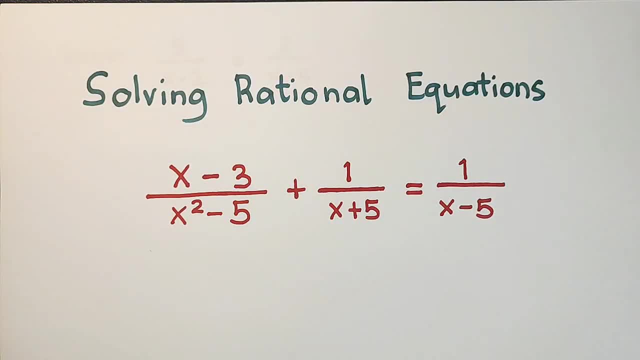 Hi guys, it's BT Chirgon. In today's video, we will talk about solving rational equations, And for this topic, or for this video tutorial, this is our main problem. So, without further ado, let's do this topic. So before we solve this problem, let us solve first an easier problem. 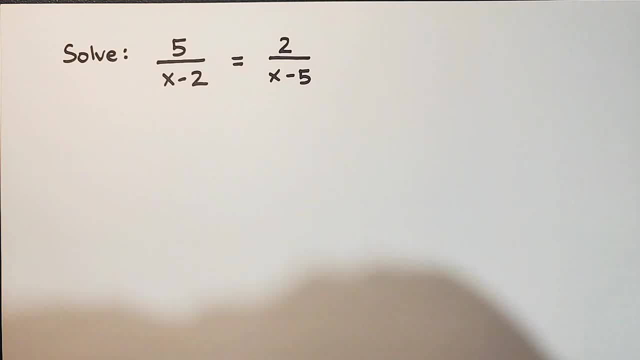 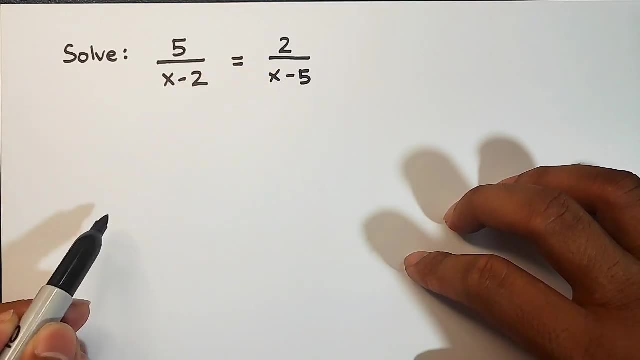 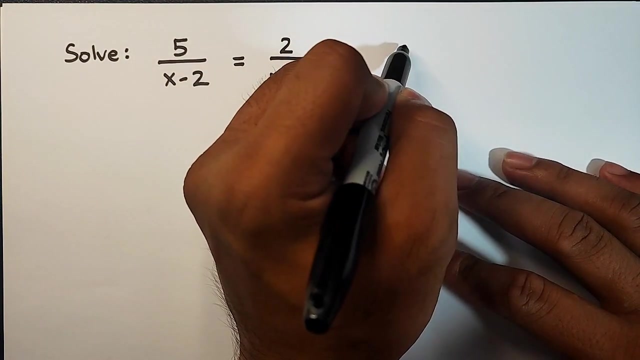 about solving rational equations. So, as you can see, we have here the first equation: 5 over x minus 2 is equal to 2 over x minus 5.. The key thing here on how to solve this equation is you need to determine your LCD first. So, as you can see, we have here: 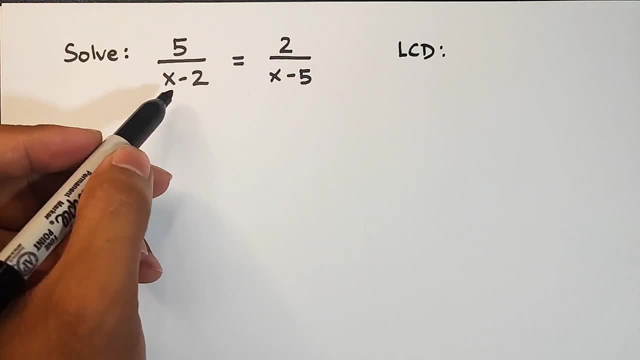 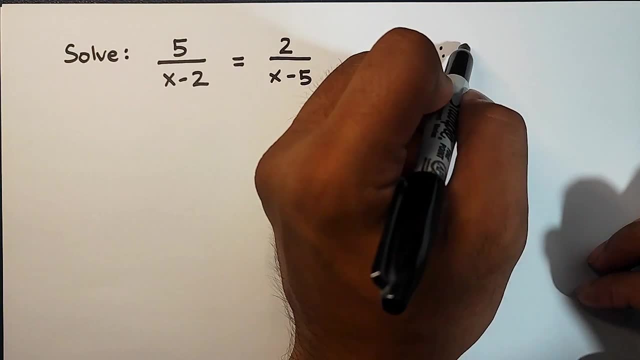 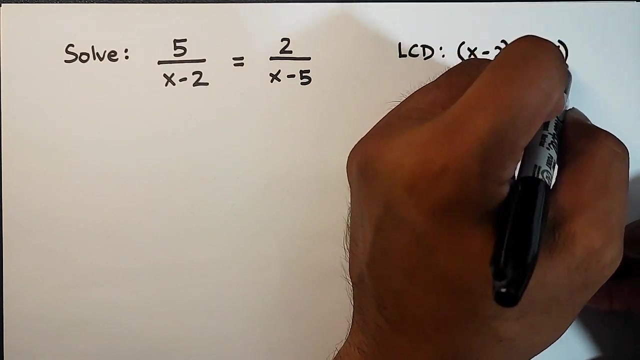 denominators x minus 2 and x minus 5.. So if you want to determine the LCD of these two denominators, simply express them as factors, like this: one x minus 2 times x minus 5.. So, as you can see, we expressed it as factors, but you don't.